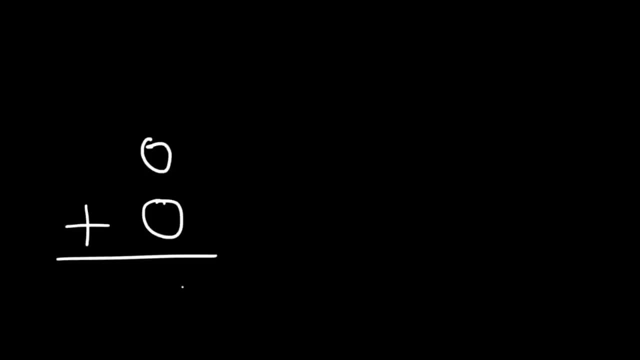 What's 0 plus 0?? 0 plus 0 is 0.. Now what about 1 plus 0?? How can we add those two binary numbers? 1 plus 0 is 1.. Now there's some other basic rules to go over. What about 1 plus 1?? 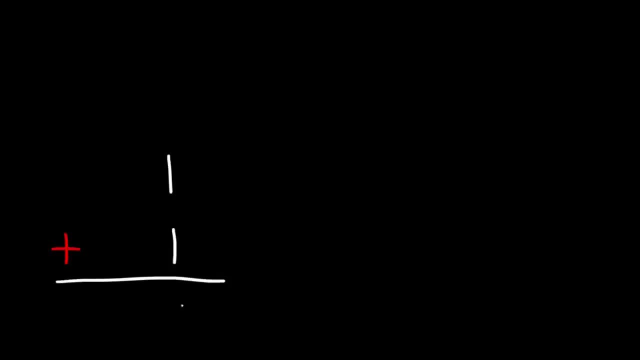 In this case we need to carry over 1 plus 1 is going to be 0, but you need to carry over a 1. And so you get 1, 0.. So basically, 1, 0 has the decimal equivalent of 2.. 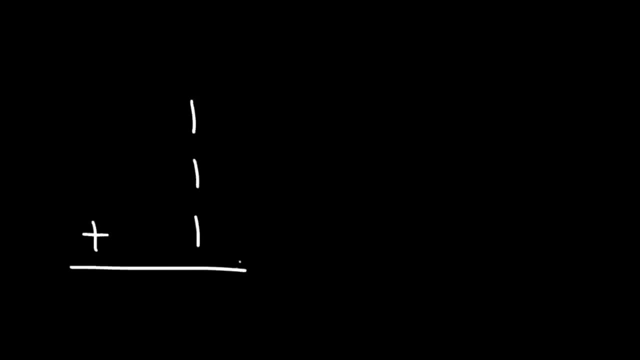 Now what if you have three 1s? How can you add this? In this case, it's going to be 1, and you carry over a 1.. Let's write that here, And so you get 1, 1.. 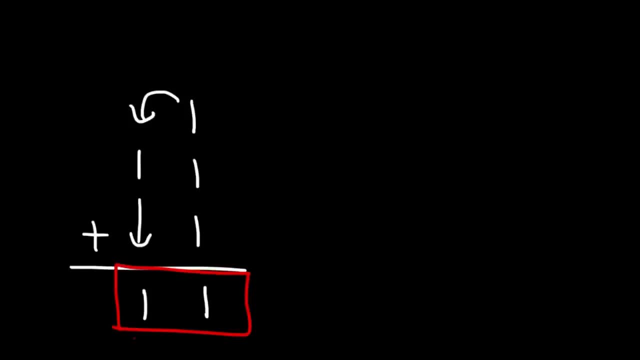 So if you have three 1s in a single column, it's going to produce an output of 1, 1.. Now let's work on some example problems. Go ahead and add these two binary numbers 1, 0, 1, 0 plus 1, 0, 0, 1.. 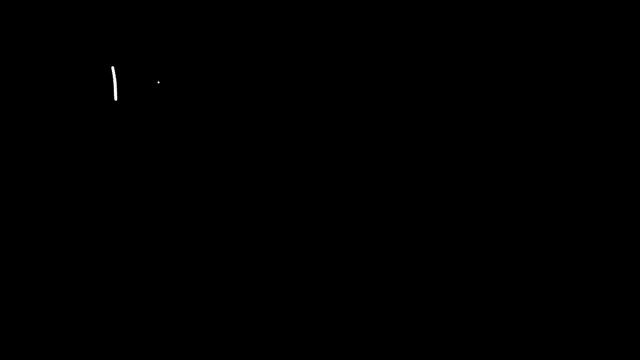 Now the first thing you should do is you should line up these numbers And then add up the numbers column by column. So here we have 0 plus 1, which is 1.. In the next column, we have 1 plus 0, which is also 1.. 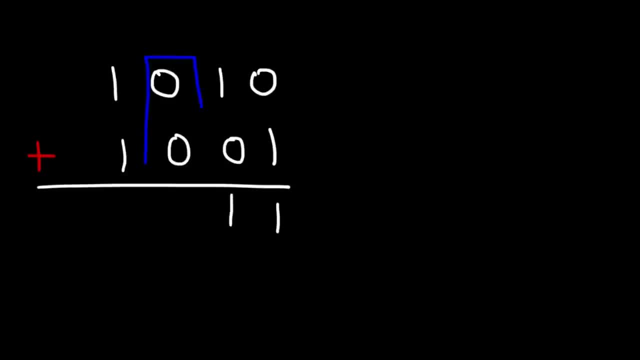 And then for the third column, 0 plus 1, I mean, that's 0 plus 0, rather, which is 0.. And then for the last one, it's 1 plus 1, which is going to be based on the last two examples, 0.. 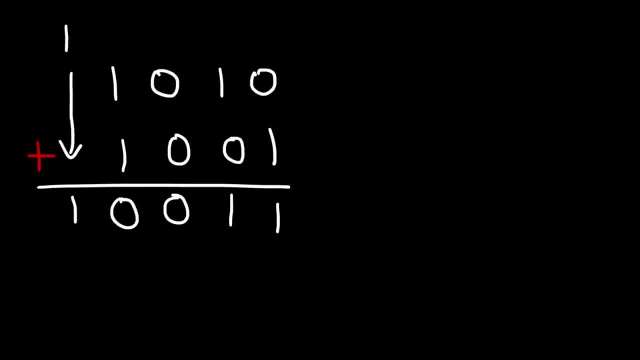 But you need to carry over a 1,, so you get 1, 0.. Now, to check the work, let's convert each binary number into one. So we're going to do a decimal number. So let's separate this into columns. 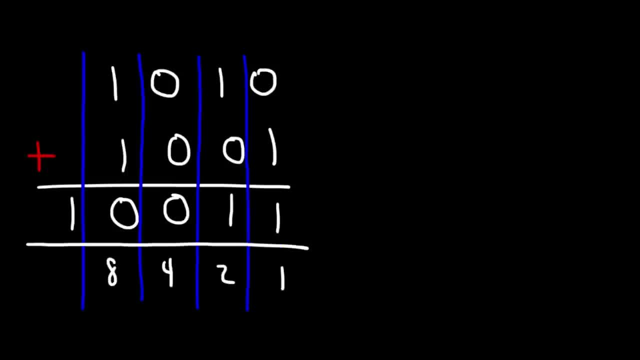 So this is 1,, 2,, 4,, 8, and 16.. So 1, 0, 1, 0 is going to have. the decimal equivalent of this is going to be 8 plus 2.. 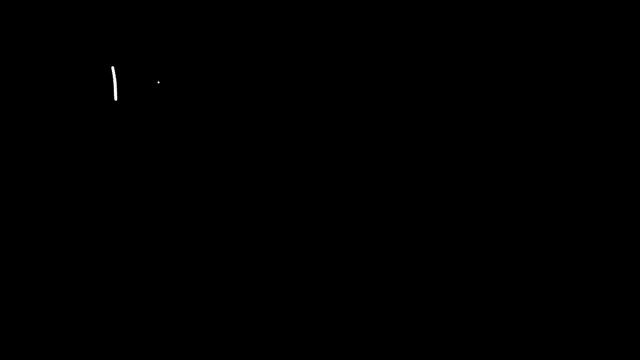 Now the first thing you should do is you should line up these numbers And then add up the numbers column by column. So here we have 0 plus 1, which is 1.. In the next column, we have 1 plus 0, which is also 1.. 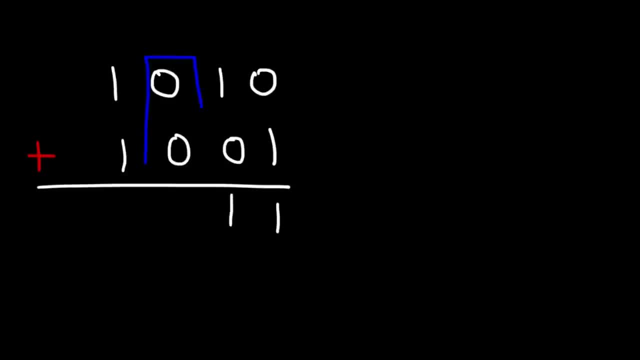 And then for the third column, 0 plus 1, I mean, that's 0 plus 0, rather, which is 0.. And then for the last one, it's 1 plus 1, which is going to be based on the last two examples, 0.. 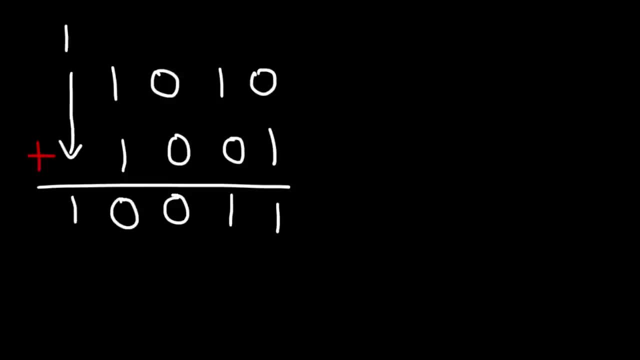 But you need to carry over a 1,, so you get 1, 0.. Now, to check the work, let's convert each binary number into one. So let's do that. So let's do a decimal number. So let's separate this into columns. 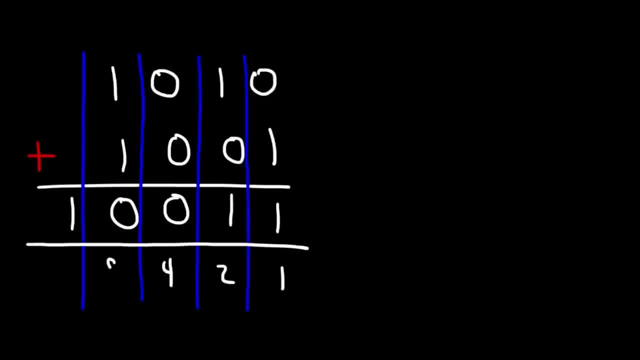 So this is 1,, 2,, 4,, 8, and 16.. So 1, 0, 1, 0 is going to have. the decimal equivalent of this is going to be 8, plus 2, and 16.. So 1, 0, 1, 0 is going to have. the decimal equivalent of this is going to be 8, plus 2, and 16.. So 1, 0, 1, 0 is going to be 8, plus 2, because it's in this column. 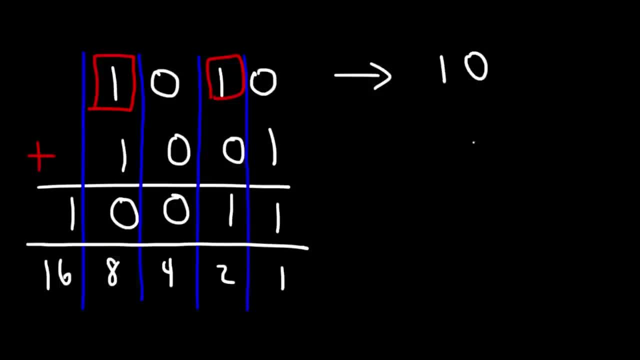 8 plus 2 is 10.. So that's the decimal equivalent of 1, 0, 1, 0.. Here we have an 8 and a 1.. So 8 plus 1 is 9.. 10 plus 9 is 19.. 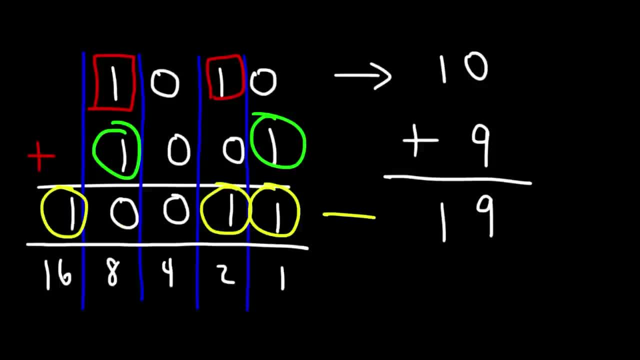 So here we have a 16 plus a 2 plus a 1.. So that adds up to 19.. And so we can see that we have the right answer. So that's the decimal equivalent of 1, 0, 1, 0.. 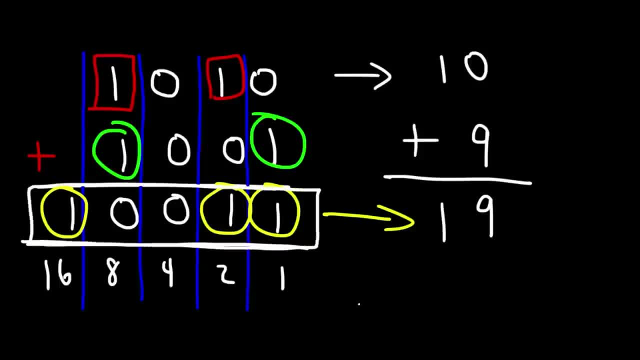 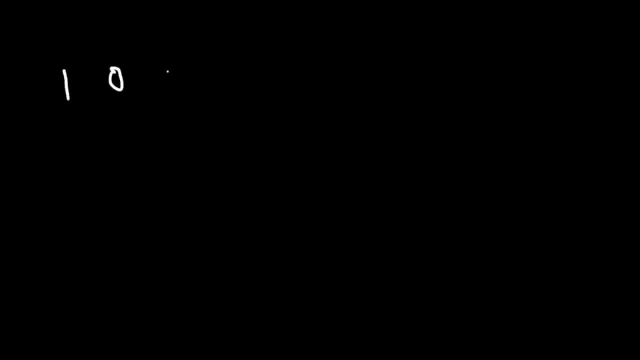 So that's the decimal equivalent of 1, 0, 1, 0.. So this is our answer right here. So that's how you can add two binary numbers. Now let's go ahead and try another example. Go ahead and add these two binary numbers. 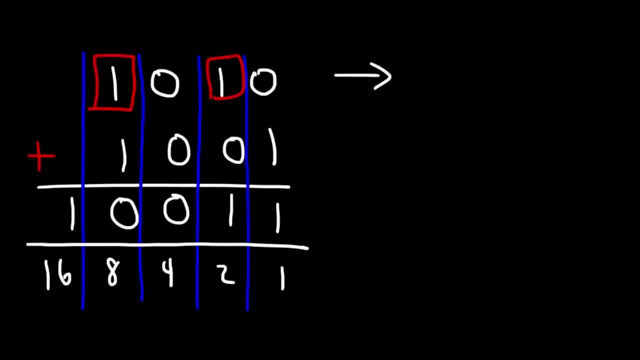 So let's separate this into columns, Because it's in this column. 8 plus 2 is 10.. So that's the decimal equivalent of 1, 0, 1, 0.. Here we have an 8 and a 1.. 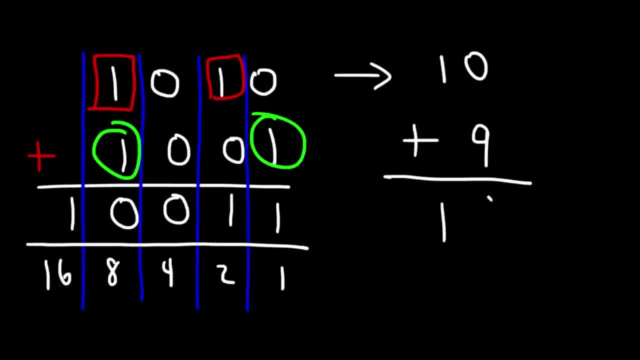 So 8 plus 1 is 9.. 10 plus 9 is 19.. So here we have a 16 plus a 2 plus a 1. So that adds up to 19.. And so we can see that we have the right answer. 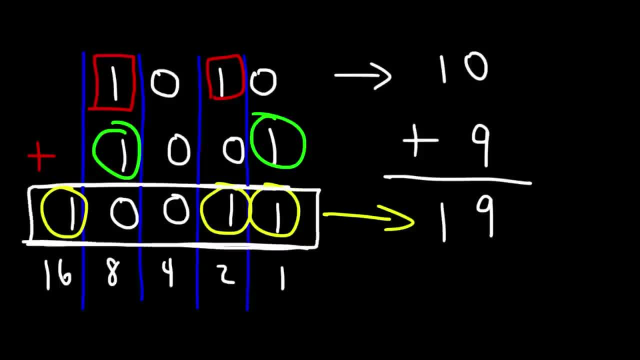 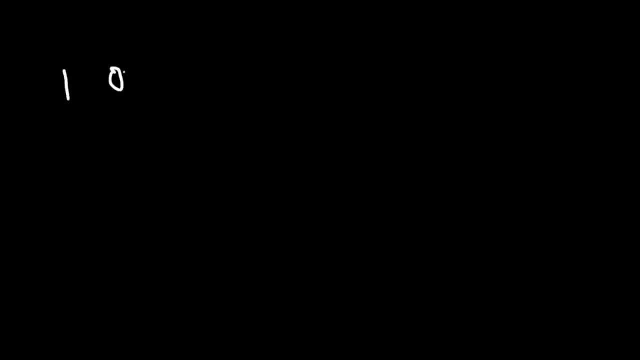 So let's do that. So this is our answer right here. So that's how you can add two binary numbers. Now let's go ahead and try another example. Go ahead and add these two binary numbers. Feel free to pause the video if you want to try this example. 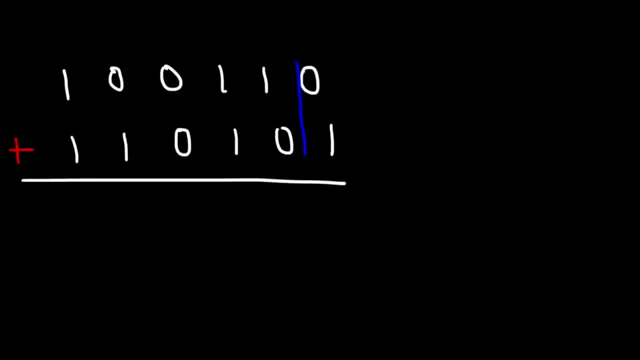 So let's start with the column on the right side: 0 plus 1 is going to be 1.. And then in the next column we have 1 plus 0,, which is 1.. And then it's 1 plus 1,, which is going to be a 0,, but we need to carry over a 1.. 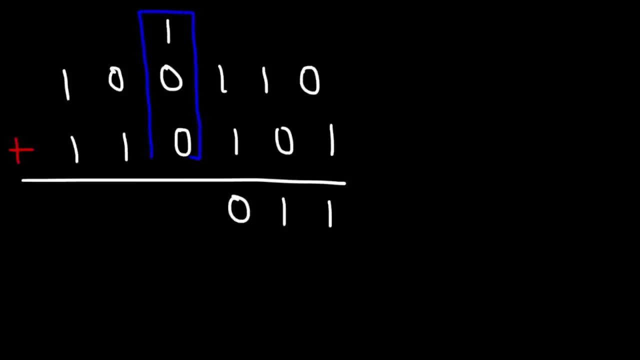 Now for the fourth column. it's 1 plus 0 plus 0, which will equal 1.. And then we have 0 plus 1., Which is 1.. And then next is 1 plus 1, which is 0, but carry over a 1 to the next column, which will give us 1.. 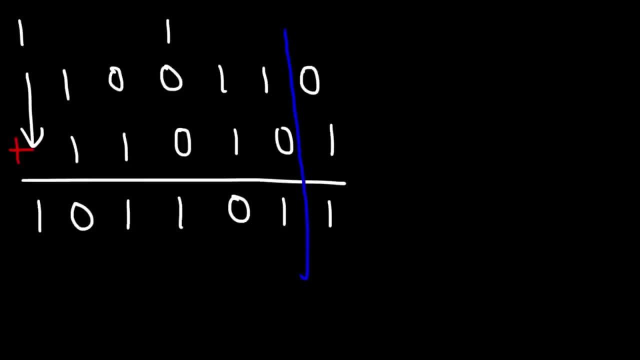 So now let's confirm our answer, But let's separate everything into columns, Just like we did before. So this is going to be 1, 2,, 4,, 8,, 16,, 32, and 64.. So let's get the decimal equivalent of the first number. 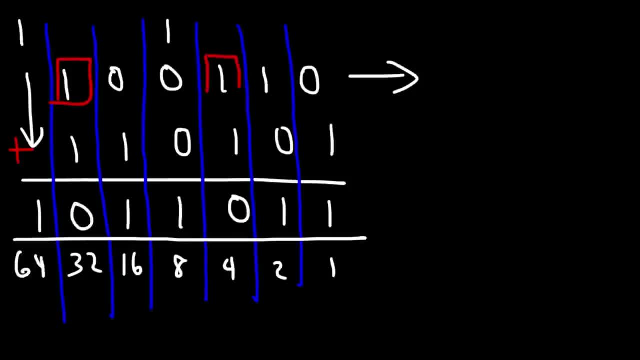 So we have a 32 plus a 4 plus a 2.. 32 plus 4 is 36, plus 2,, that's 38. And then for the next one, we have a 32 plus 16,, which is 48.. 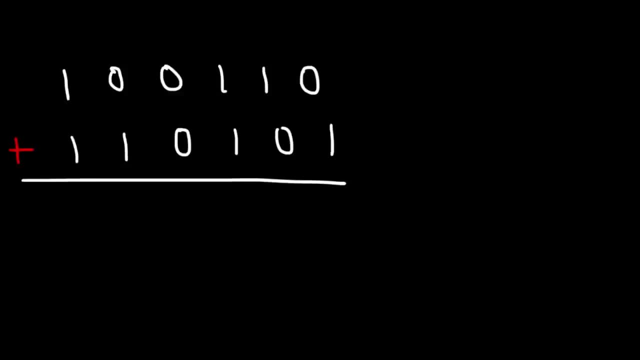 Feel free to pause the video if you want to try this example. So let's start with the column on the right side: 0 plus 1 is going to be 1.. And then in the next column, we have 1 plus 0, which is 1.. 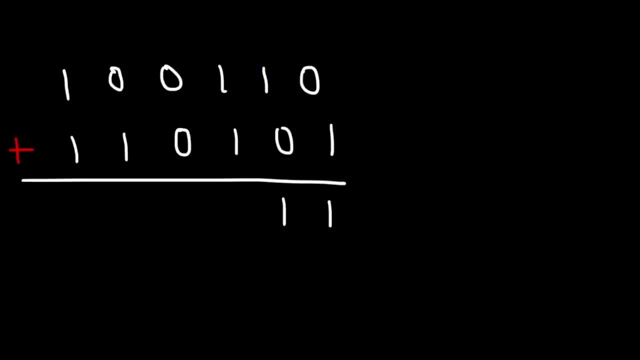 And then it's 1 plus 1,, which is going to be a 0,, but we need to carry over a 1.. Now for the fourth column. it's 1 plus 0 plus 0, which will equal 1.. 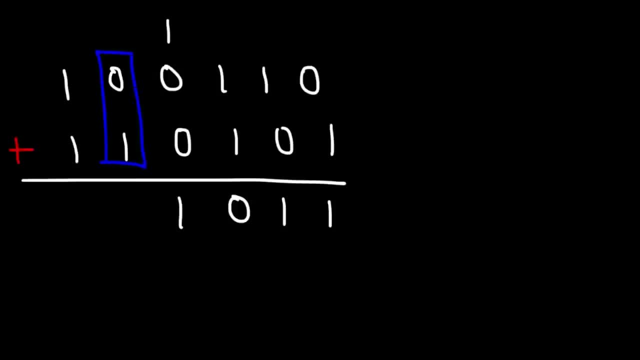 And then we have 0 plus 1. Which is 1.. And then next is 1 plus 1,, which is 0, but carry over a 1 to the next column, which will give us 1.. So now let's confirm our answer. 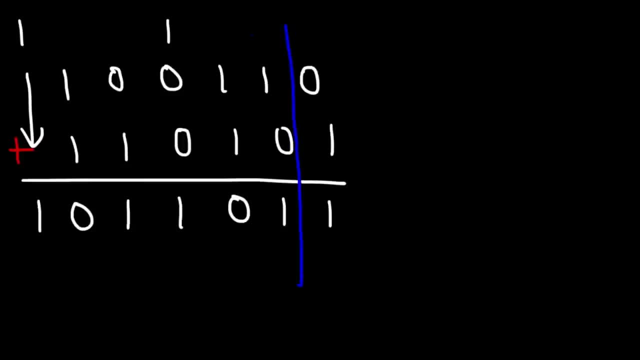 But let's separate everything into columns, Just like we did before. So this is going to be 1,, 2,, 4,, 8,, 16,, 32, and 64.. So let's get the decimal equivalent of the first number. 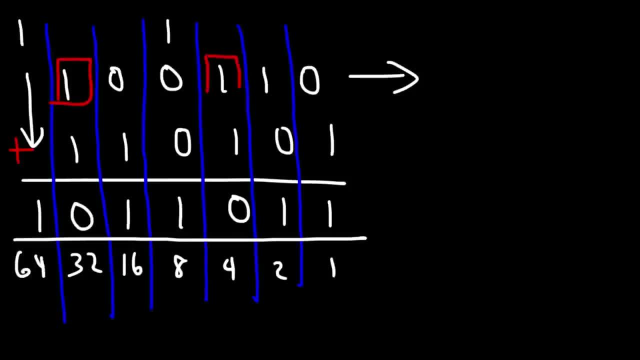 So we have a 32 plus a 4 plus a 2.. 32 plus 4 is 36, plus 2,, that's 38. And then for the next one, we have a 32 plus 16,, which is 48.. 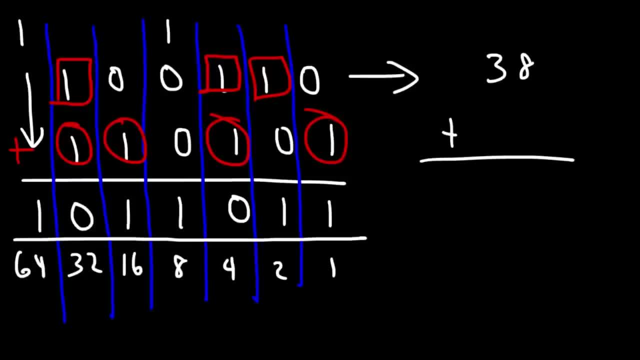 48 plus 4 is 52, plus 1.. That's going to be 53.. Now, 8 plus 3 is 11,. carry over the 1.. 5 plus 3 is 8, plus 1, that's 9.. 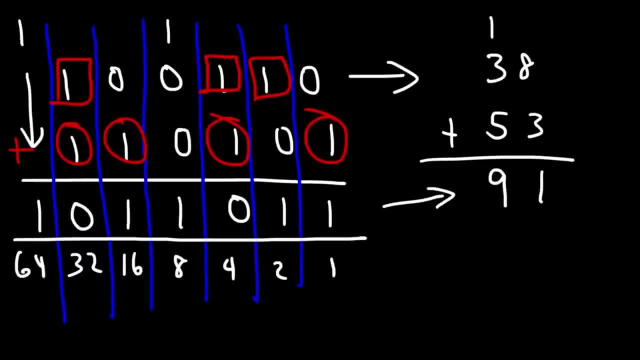 So this should equal 91.. So we have a 64 plus 16,, so that's 80, plus 8,, that's 88.. Plus 2 is 1.. Plus 1 is 90,, plus 1, 91.. 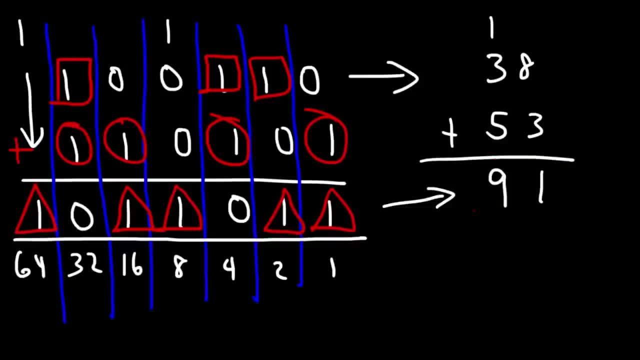 So we can see that we do indeed get the right answer. And so now you know how to add binary numbers. As you can see, it's not very difficult as long as you follow the process. So make sure you remember these two things. 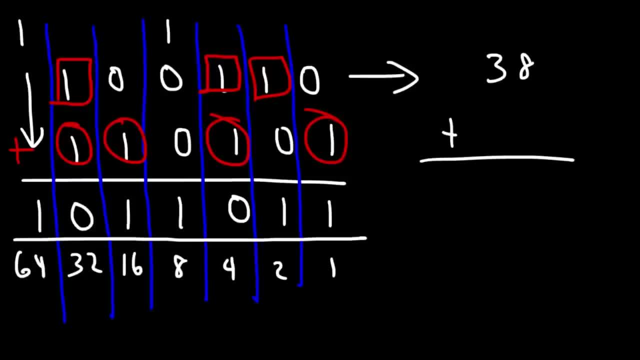 48 plus 4 is 52, plus 1.. That's going to be 53.. Now, 8 plus 3 is 11,. carry over the 1.. 5 plus 3 is 8, plus 1, that's 9.. 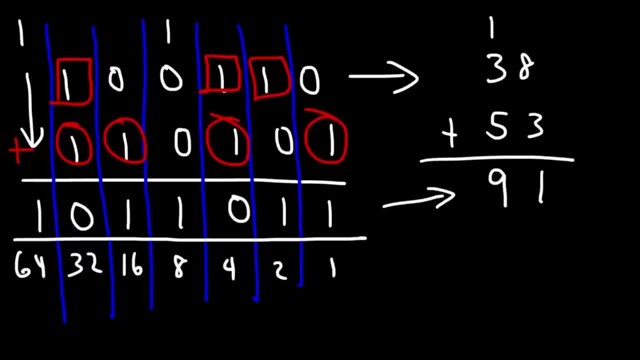 So this should equal 91.. So we have a 64 plus 16,, so that's 80, plus 8,, that's 88.. Plus 2 is 1. 90 plus 191.. So we can see that we do indeed get the right answer. And so now you know. 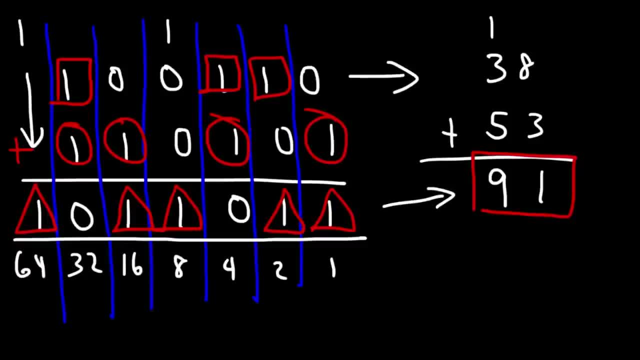 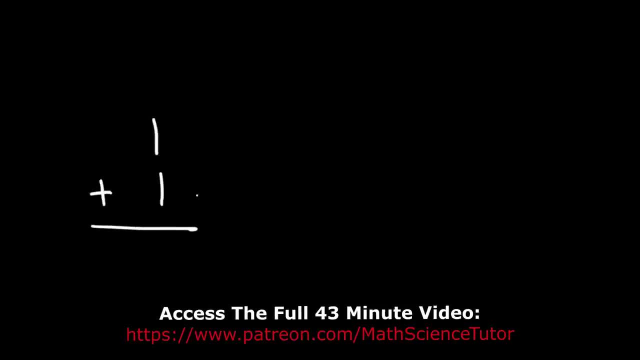 how to add binary numbers. As you can see, it's not very difficult as long as you follow the process. So make sure you remember these two things. When adding 1 plus 1, you're going to get a 0, but you need to carry over a 1 to the next column, And so the end result. 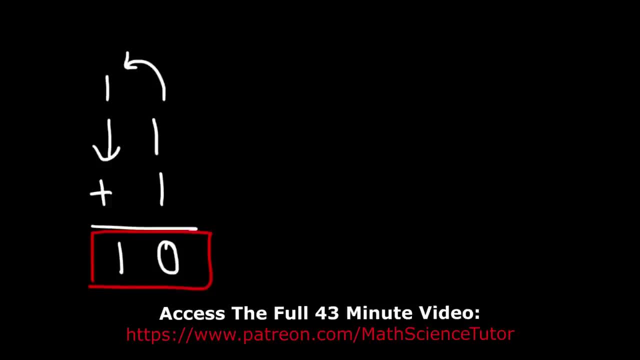 is that you get 1, 0. And if you're adding three 1s together, it's going to be 1, but you carry over another 1.. And so instead of getting 1, 0,, you get 1, 1.. And if you remember, 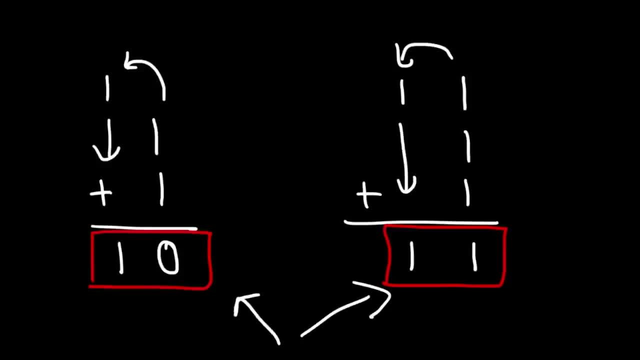 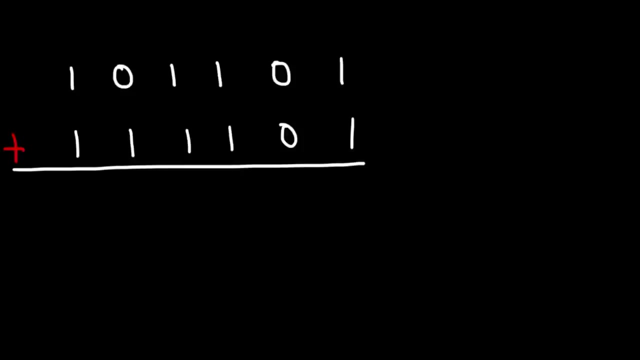 these two things. you can easily add two binary numbers together. For the sake of practice, let's work on another example. So go ahead and add these numbers. So feel free to take a minute, pause the video and work on this example problem. So let's start from the first column on the right side and 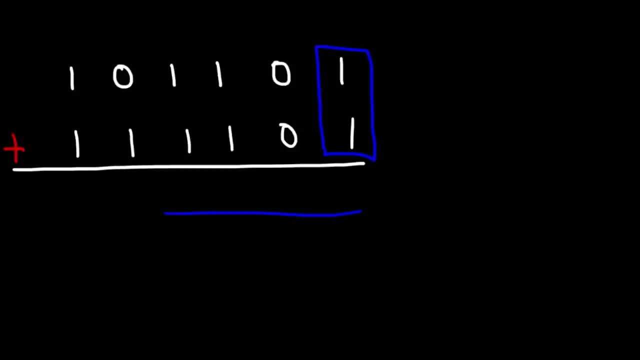 work our way towards the left. One plus one. we know that it's going to give us 0,, but we need to carry over one, And so we're going to add two binary numbers together. So let's over a 1 to the next column. 1 plus 0 plus 0 is going to be 1, and then in the third: 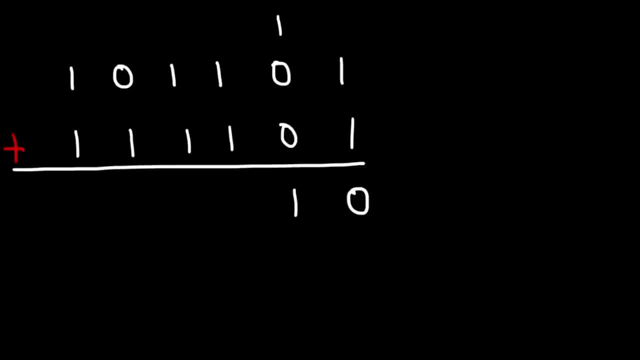 column we have 1 plus 1, which is 0, but we got to carry over a 1.. Now for the fourth column. we have three 1s. Do you remember what we need to do if we encounter this situation? If you have three 1s in a single column, it's going to give you a 1 for that column, but 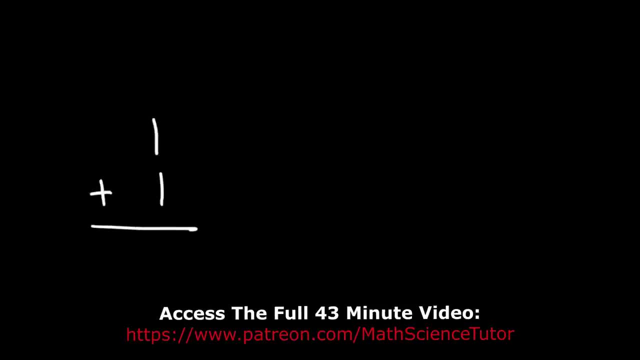 When adding 1 plus 1,, you're going to get a 0,, but you need to carry over a 1 to the next column, And so the end result is that you get 1, 0.. 1, 0.. 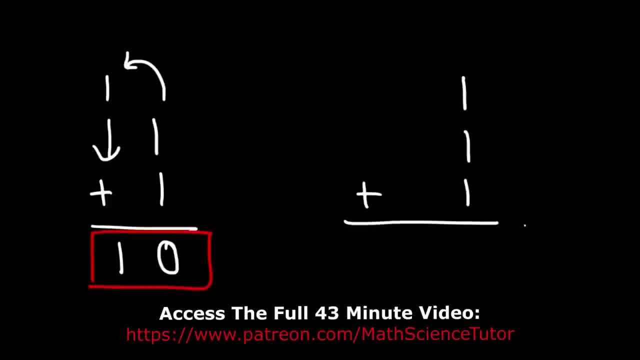 And if you're adding three 1s together, it's going to be 1,, but you carry over another 1.. And so instead of getting 1, 0,, you get 1, 1.. And if you remember these two things, you can easily add two binary numbers together. 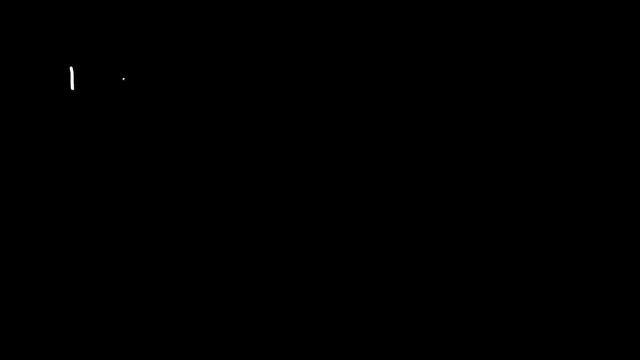 For the sake of practice, let's work on another example. So go ahead and add these numbers. So feel free to take a minute, pause the video and work on this example problem. So let's start from the first column on the right side and work our way towards the left. 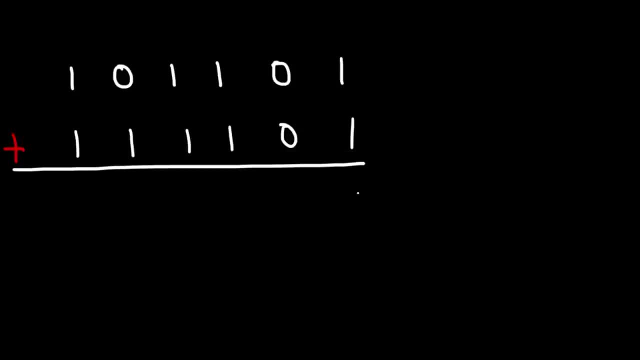 1 plus 1, we know that it's going to give us 0, but we need to carry over a 1 to the next column. 1 plus 0 plus 0 is going to be 1.. And then in the third column, we have 1 plus 1, which is 0, but we've got to carry over a 1.. 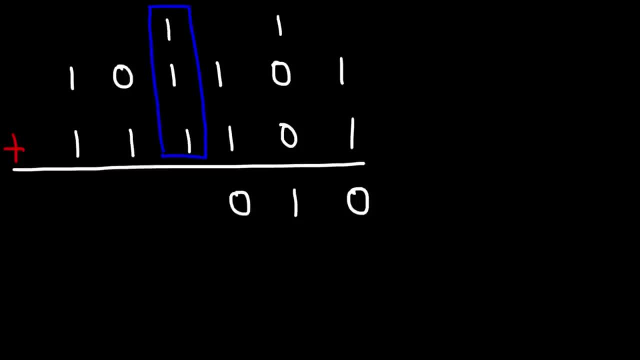 Now for the fourth column. we have three 1s. Do you remember what we need to do if we encounter this situation? If you have three 1s in a single column, it's going to give you a 1 for that column. 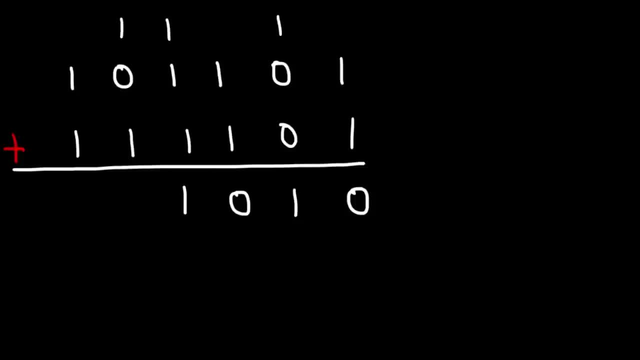 but you need to carry over another 1.. So 1 plus 0 plus 1 is going to give us 0,, but we need to carry over a 1 to the next column, And so 1 plus 0 plus 1, we could ignore the 0, and so it's the same as 1 plus 1,. 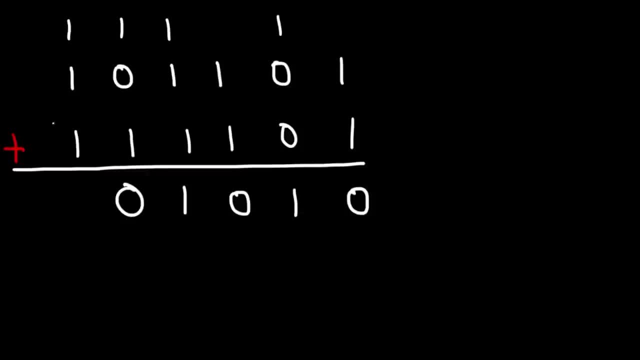 which will give us a 0 for that column, but we've got to carry over a 1.. And for the last column we have three 1s again. so it's going to produce a 1 for that column, but we need to carry over another 1 for the next column. 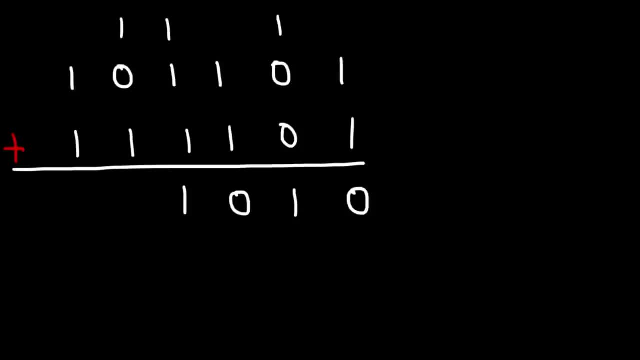 you need to carry over another 1 to the next column, And so 1 plus 0 plus 1, we could ignore the 0, and so it's the same as 1 plus 1,, which will give us a 0 for that column. but we got. 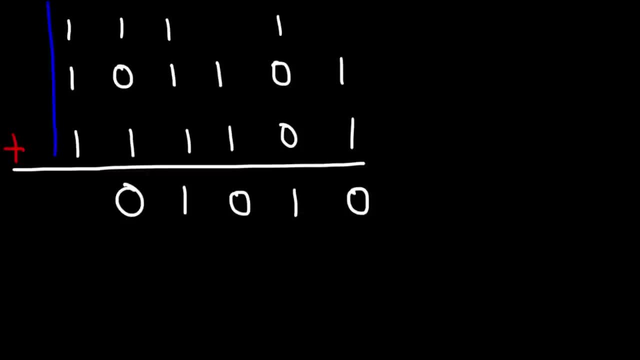 to carry over a 1.. And for the last column we have three 1s again, so it's going to produce a 1 for that column, but we need to carry over another 1 for the next column. So 1 plus 0 plus 1 is going to be 1.. And if you have three 1s in a single column it's going. 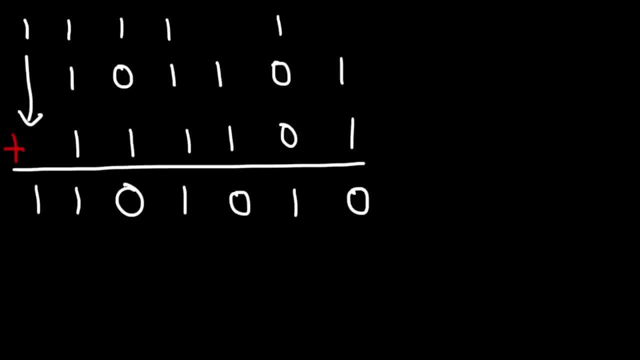 plus nothing, it's going to give us one, and so this here is our final answer, but, as always, let's confirm it. so let's begin by drawing lines to separate the columns from each other, and then let's write the powers of two. two to zero is 12 to the one is 22. 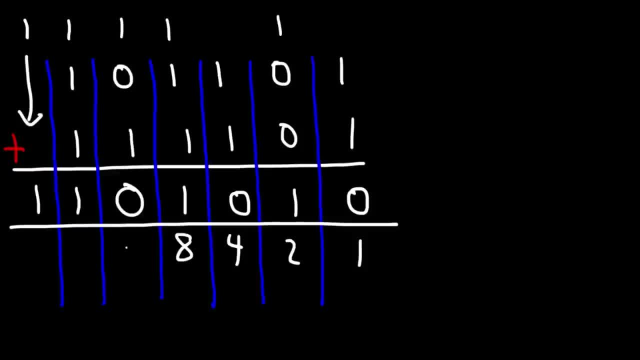 squared is 42 to the third power is 82, to the fourth power 16. to the fifth is 32, and 2 to 6 is 64. so let's convert the first binary number into its decimal equivalent. so we have a 32 plus 8. 32 plus 8 is 40 plus 4, that's 44 plus 1, so that's a. 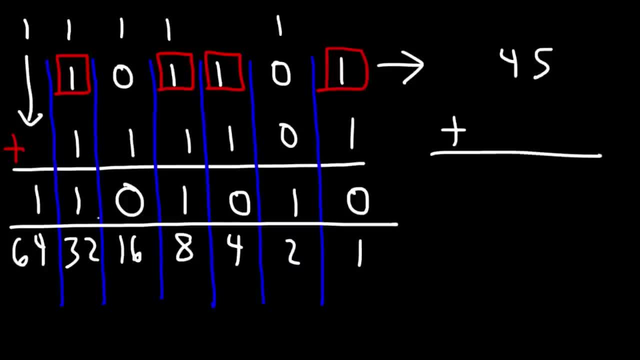 total of 45. next we have a 1 for the 32 columns. that's 32 plus 1 for the 16 column. so 32 plus 16, that's 48 plus 8, that's 56 plus 4, that's 60 plus 1, and so that's going to be 61. now, 1 plus 5 is 64 plus 6. 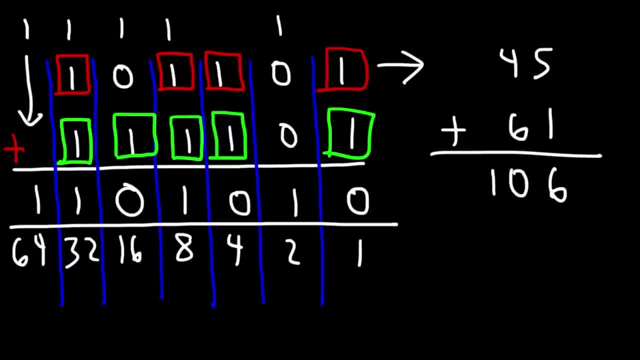 is 10, so we get 106. now we have a 64 plus 32, so that's 96. 96 plus 8 is a 104. 104 plus 2 is 106, and so our answer is indeed correct. so this is the final answer right here. 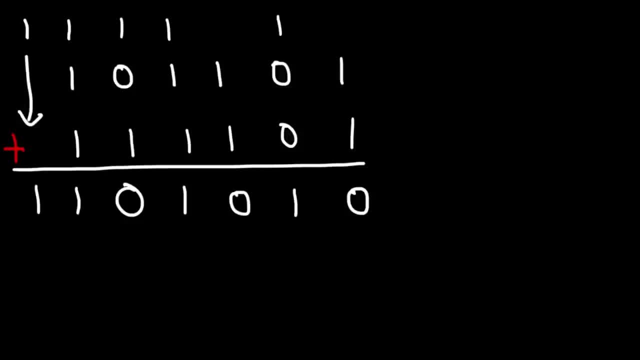 So 1 plus nothing is going to give us 1.. And so this here is our first column, Final answer. But as always, let's confirm it. So let's begin by drawing lines to separate the columns from each other, And then let's write the powers of 2.. 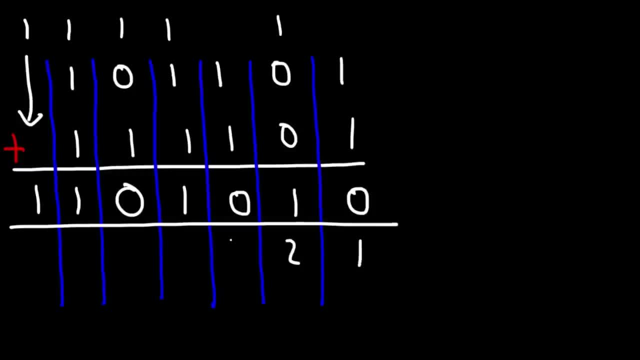 2 to the 0 is 1.. 2 to the 1 is 2.. 2 squared is 4.. 2 to the third power is 8.. 2 to the fourth power is 16.. 2 to the fifth is 32.. 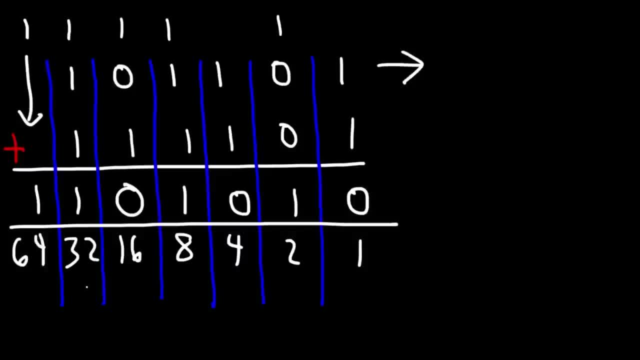 And 2 to the sixth is 64. So let's convert the first binary number into its decimal equivalent, So we have a 32 plus 8.. 32 plus 8 is 40. Plus 4,, that's 44, plus 1.. 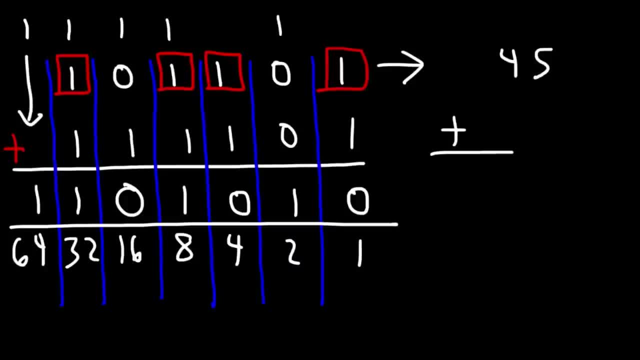 So that's a total of 45.. Next we have a 1 for the 32.. So that's 32.. Plus a 1 for the 16th column. So 32 plus 16, that's 48, plus 8, that's 56, plus 4,, that's 60, plus 1, and so that's going to be 61.. 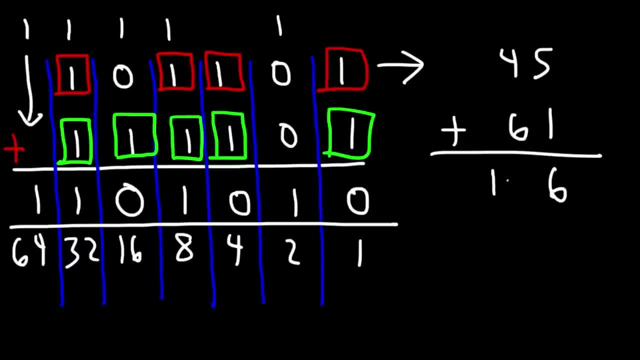 Now, 1 plus 5 is 6,, 4 plus 6 is 10. So we get 106.. Now we have a 64 plus a 32,, so that's 96.. Now we have a 64 plus a 32,, so that's 96.. 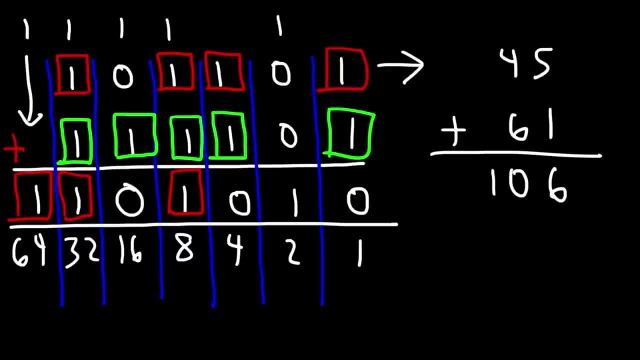 Now we have a 64 plus a 32,, so that's 96.. 96 plus 8 is 104.. 104 plus 2 is 106. And so our answer is indeed correct. So this is the final answer, right here. 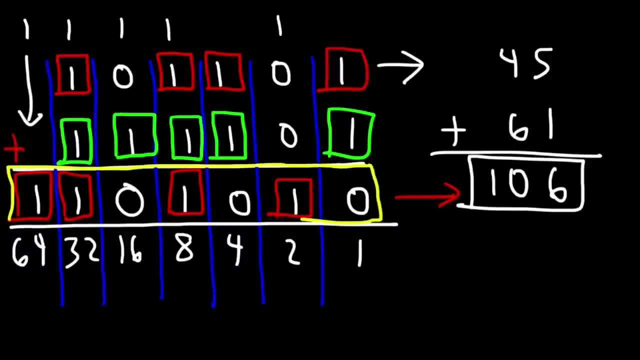 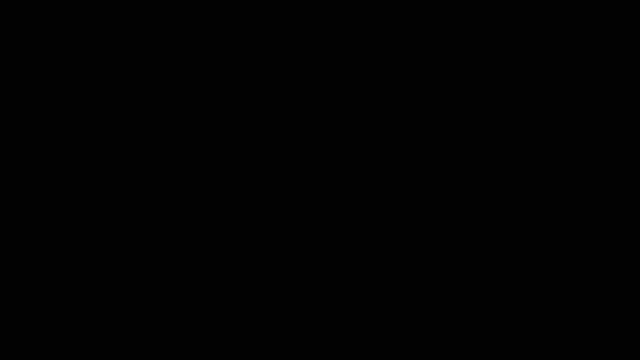 1, 1, 0, 1, 0, 1, 0.. Now let's move on to our next topic, That is, how to subtract binary numbers. So let's start with this: What is 1 minus 0?? 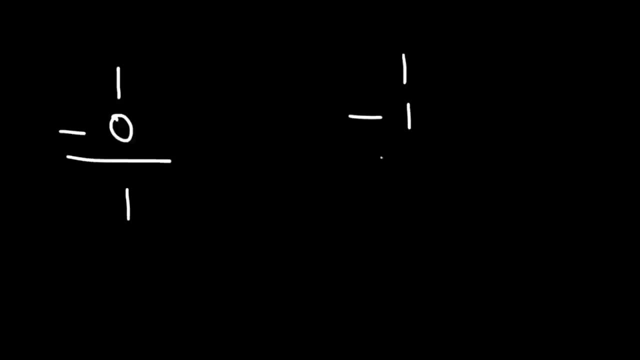 1 minus 0 is simply 1.. Now what about 1 minus 1?? 1 minus 1,, they cancel and that's 0.. Now what if you have 1, 0, but you wish to subtract it by 1?? 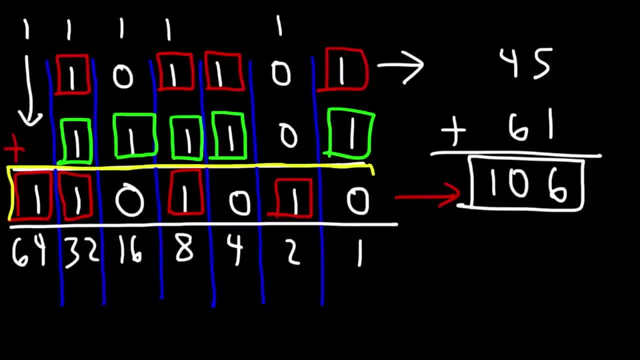 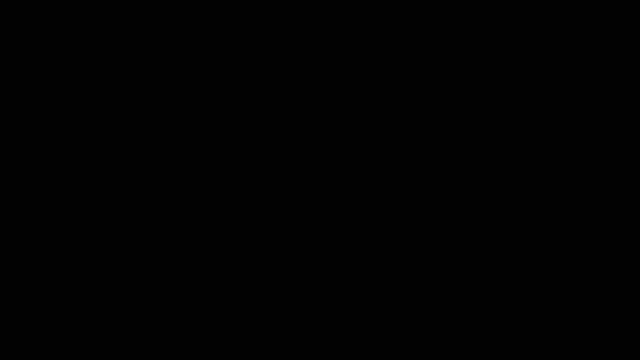 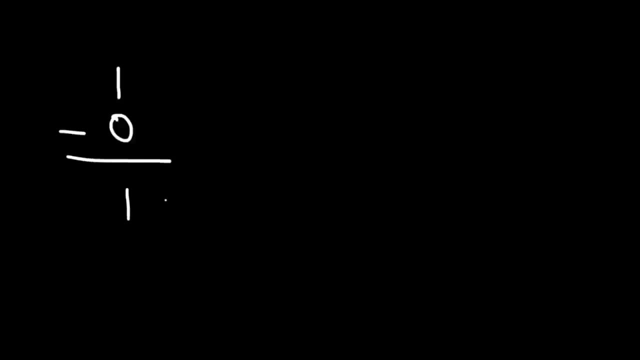 one, one, zero, one, zero, one, zero. now let's move on to our next topic, that is, how to subtract binary numbers. so let's start with this: what is 1 minus 0? 1 minus 0 is simply 1. now what about 1 minus 1? 1 minus 1: they cancel, and that's 0. now what if you have 1 minus 1? they cancel and that's 0. now what if you have 1 minus 1? they cancel and that's 0. now what if you have? 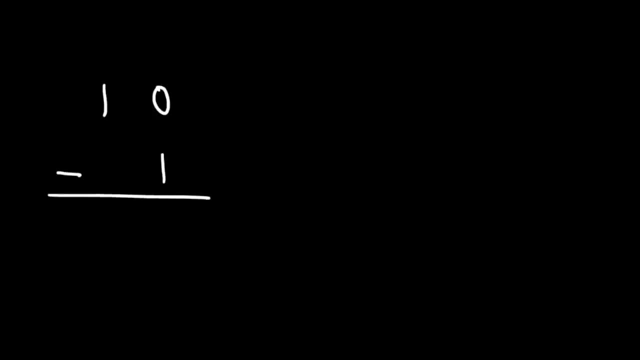 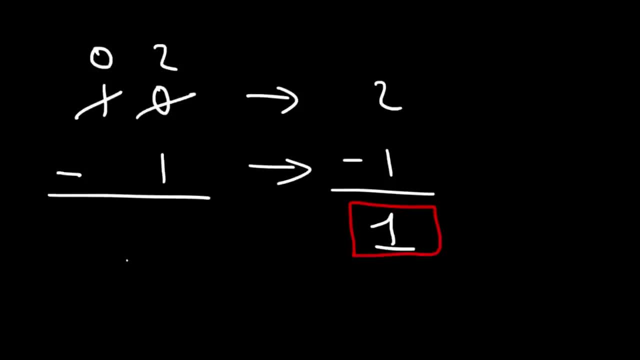 into a 0, and then this 0 becomes a 2.. 2 minus 1 is 1, and 0 minus nothing is 0. So 0, 1 corresponds to 1.. Now what if we have this situation? Let's say it's 1, 0, 0 minus 1, 0.. Now this column is: 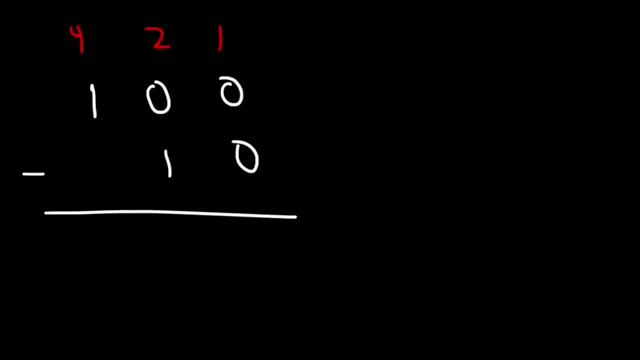 for the 1s, 2, and 4.. So 1, 0, 0 is basically 4, and 1, 0 is 2.. 4 minus 2 is 2.. So this is the answer we should get, Starting with the first column: 0 minus 0 is 0.. Now 0 minus 1, we can't. 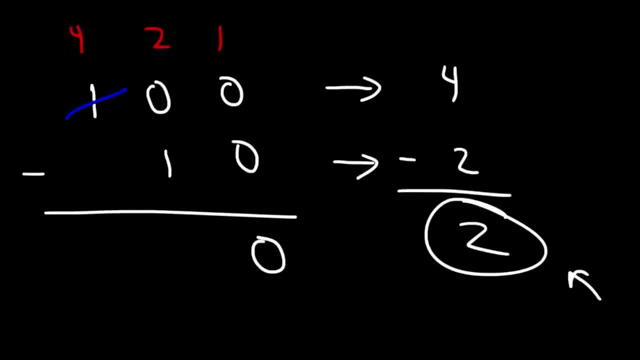 do that, so we need to borrow a 1.. So that's going to disappear, that's going to change to 0, and this becomes a 2.. 2 minus 1 is 1., And you could bring the 0 down if you want to 0, 1, 0 has the decimal equivalent of 2,. 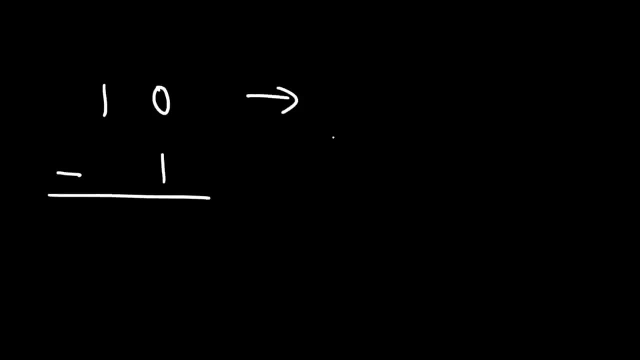 What will you do Now? 1,- 0, as a binary number, is equivalent to 2 in the decimal system And 1 is just 1 in the decimal system. So 2 minus 1 should give us 1.. 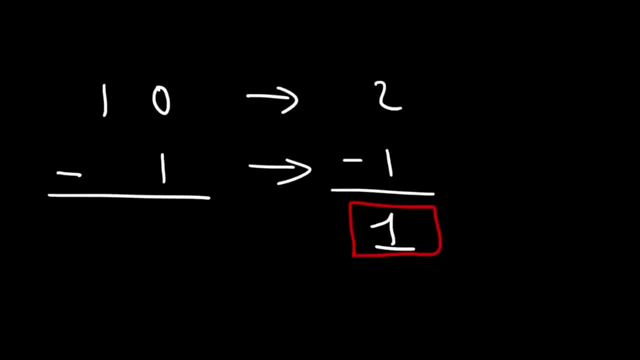 Now we can't do 0 minus 1, because that's going to give us a negative number. so we need to borrow. So we're going to borrow this 1, that's going to turn into a 0, and then this 0 becomes. 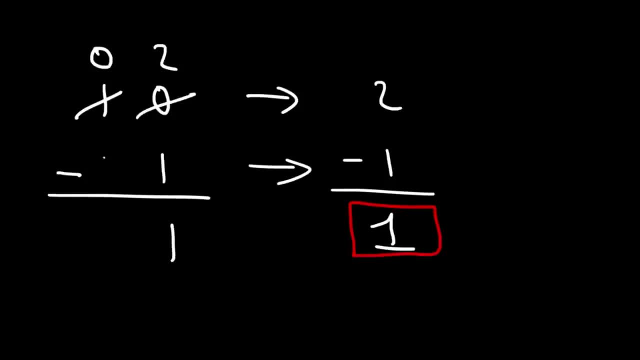 a 2.. 2 minus 1 is 1. And 0 minus nothing is 0.. So 0, 1 corresponds to 1.. Now what if we have this situation? Let's say it's 1 minus 0.. 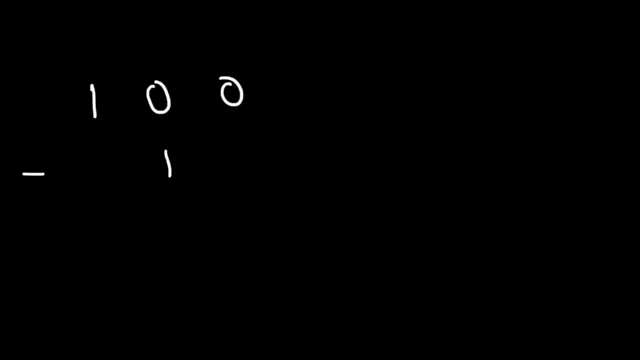 What would that mean? 0, 0 minus 1, 0.. Now this column is for the 1's, 2 and 4.. So 1, 0, 0 is basically 4 and 1, 0 is 2.. 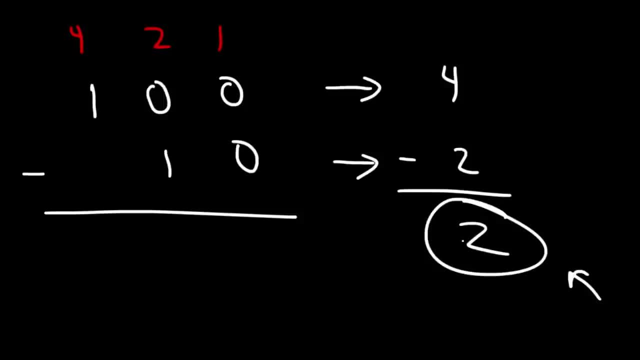 4 minus 2 is 2.. So this is the answer we should get, Starting with the first column: 0 minus 0 is 0.. Now 0 minus 1, we can't do that, so we need to borrow a 1.. So that's going to. 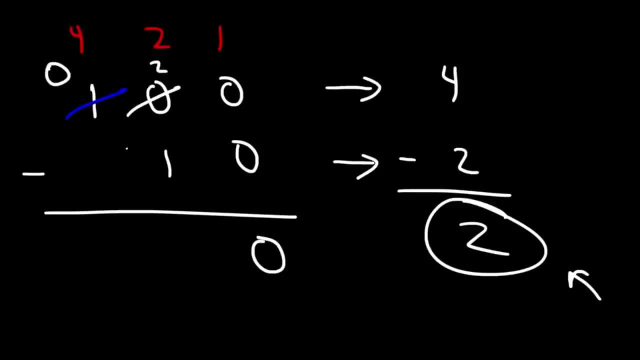 disappear. that's going to change to 0, and this becomes a 2.. 2 minus 1 is 1., And you could bring the 0 down if you want to 0,. 1, 0 has the decimal equivalent of 2,, so this: 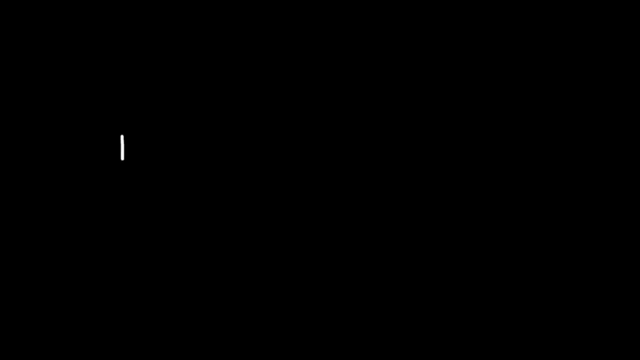 answer is correct. Now let's try this one: 1, 0,, 0 minus 1.. Go ahead and subtract those two binary numbers. So we can't do the first column. 0 minus 1 will give us a negative number, so we need to borrow a 1.. Now we can't borrow anything from this column. 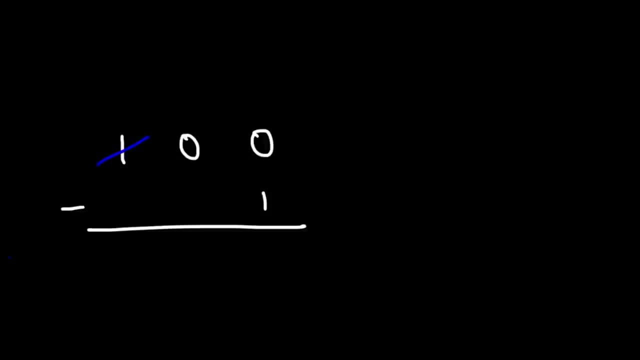 because it's a 0. So we need to borrow a 1 from a column that has a 1.. So this becomes a 0, and this column becomes a 2.. So anytime you cross out a 0, replace it with a 2.. It's.